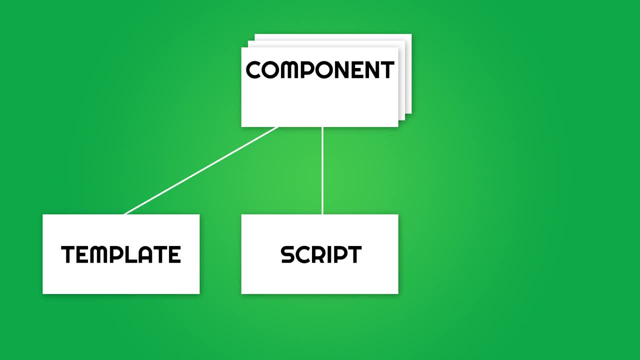 on. And the last, the third part, is for our style in this component. Now, with these three parts here- Template, script and style- we got a valid Vuejs file called a single file component, where we outsource template and script logic in a separate file. 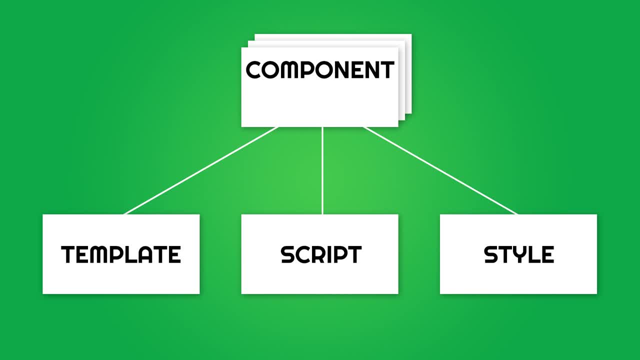 And that's one thing I love in Vuejs- These three parts are in one file and not separated and distributed over the whole application. In my opinion, that's an incredible advantage. You have, with this component structure here, Everything you need on the place. 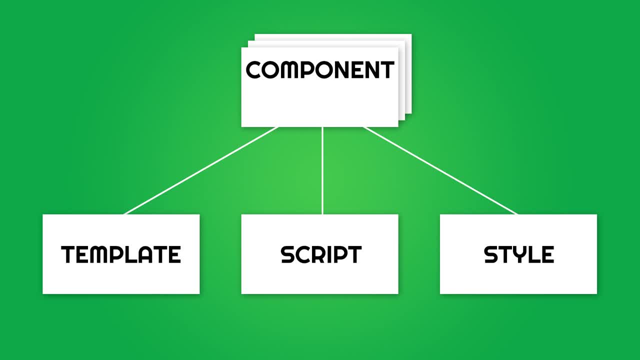 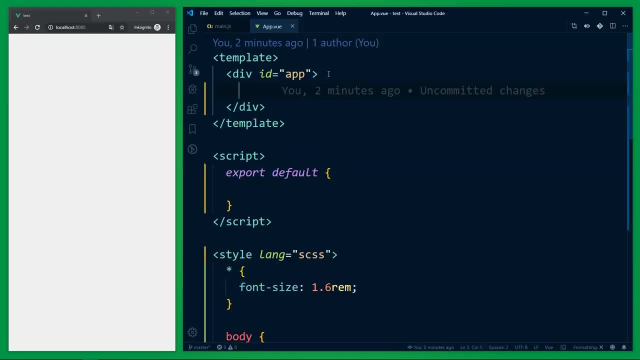 Ok, how you can use components and how you can register them. Now you will see this here in action. I'm in a brand new project here and I opened up the appvue file. By the way, this is not a conventional component. it's a separate object which we are exporting. 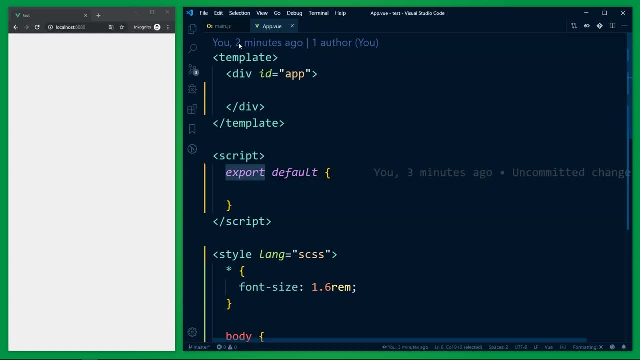 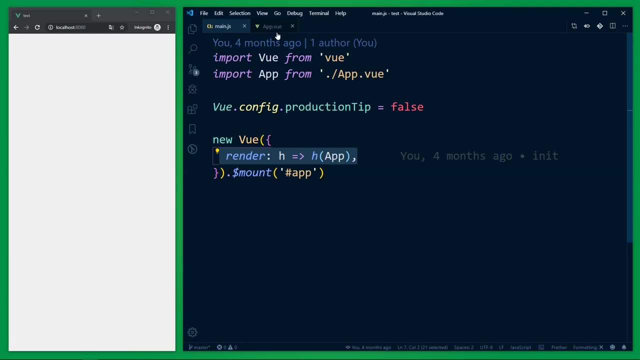 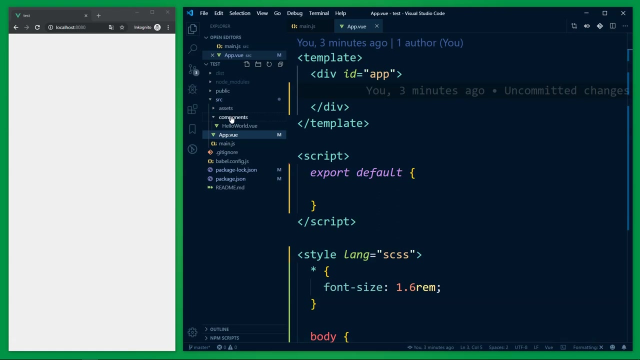 here And rendering this object at this place. This root component has the same limitations as a conventional component, but without a selector. More about that in a second. Now let's create a new component. For that I will create a new file in the components folder named statusvue. 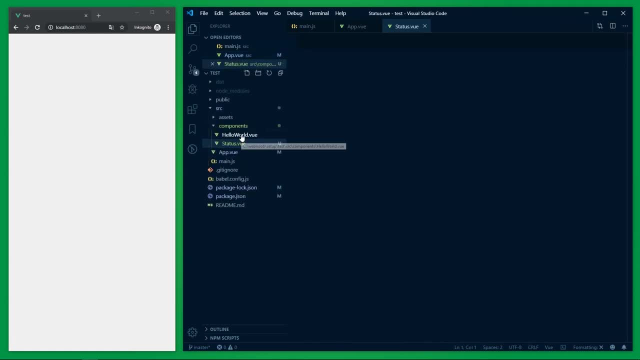 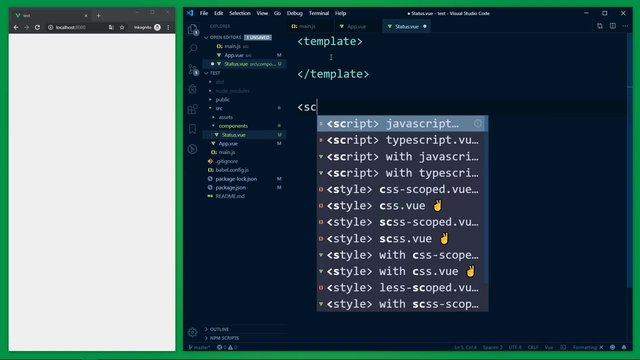 Ok, I want to delete this other hello world component here. we don't need that Now in this new component. we need a template and we need a script. We don't need style here in this case, so I leave that out. 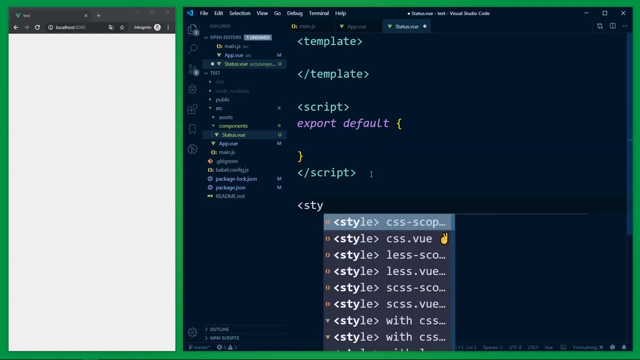 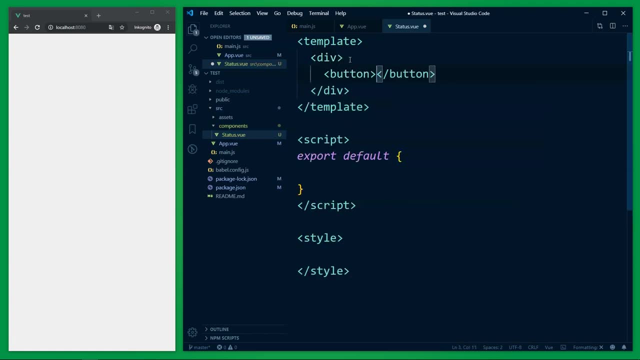 Or maybe, yes, let's place here the style section for later. Now let's stick to the template And let's create a simple button With change status as text and a click event which changes my status. After this button, I output the status. 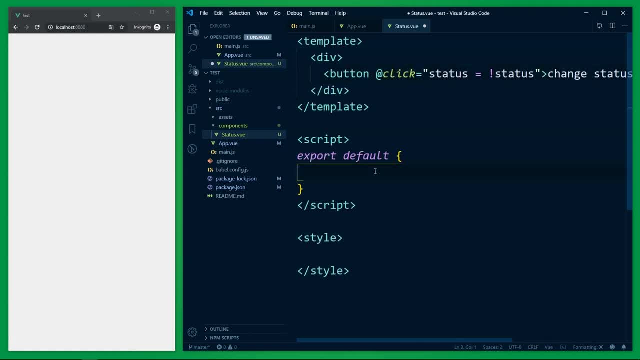 Between the script text. I want to export an object- export default, since it is the only export in this file- And here I want to have my data field, which again is a function where I return an object where status is set to false. 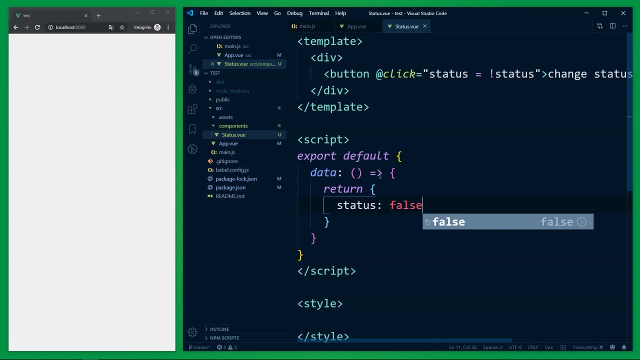 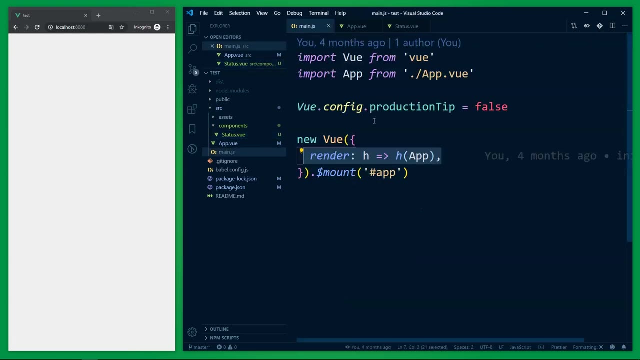 Now, with this setup, I created a component And now you can use this new component. Hmm, how you can use it? You can register it globally in the mainjs file by saying view component, giving it a selector- let's say app status, to have a unique selector. and then the object, let's 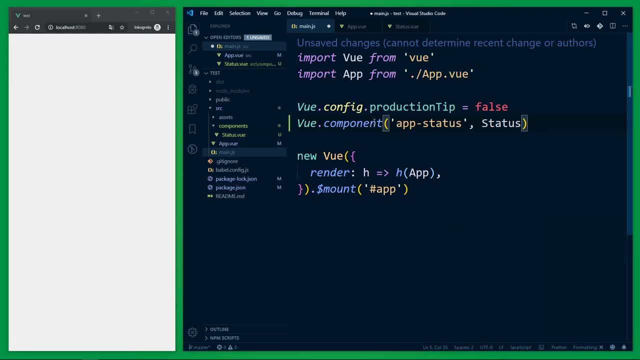 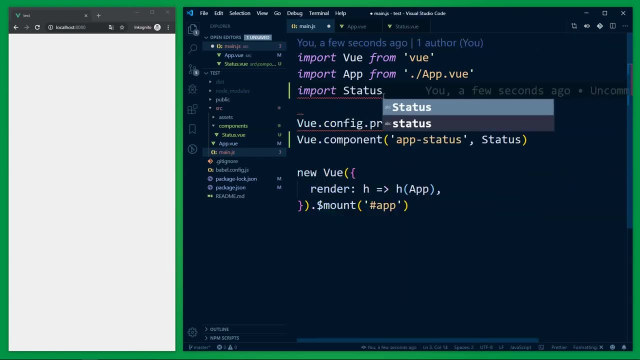 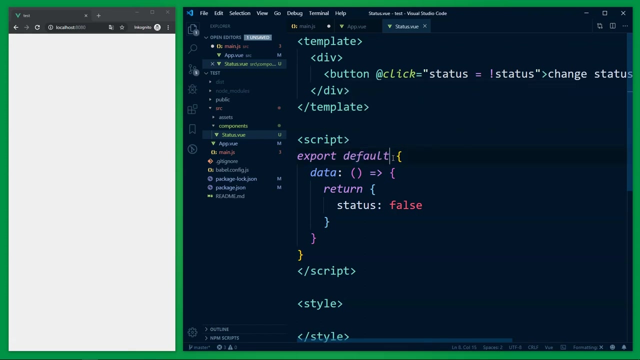 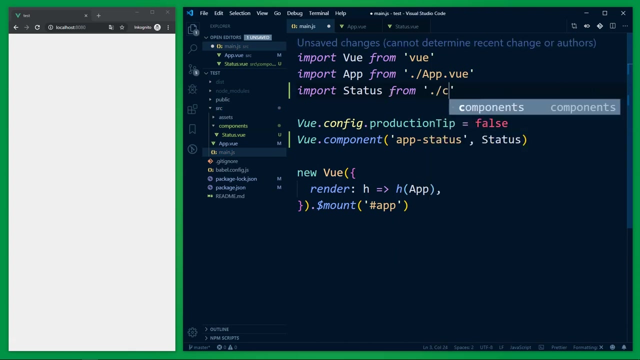 name it status. For that you need an import. I will name it status. Ok, We export only one object, export default. We don't have a name here, So you may choose any name when importing it And import it from the components folder. 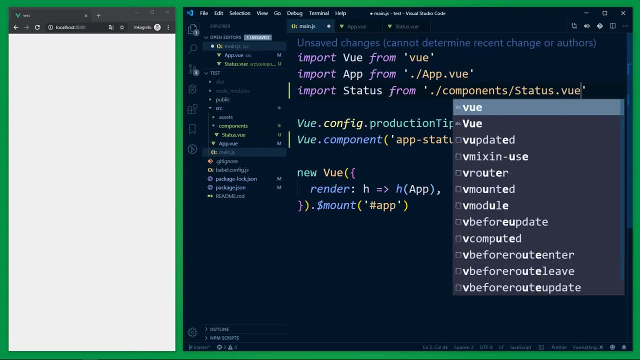 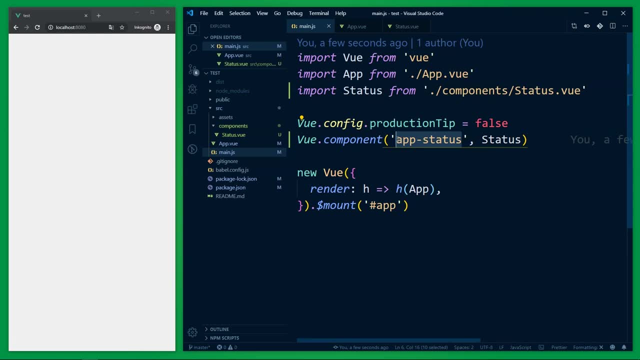 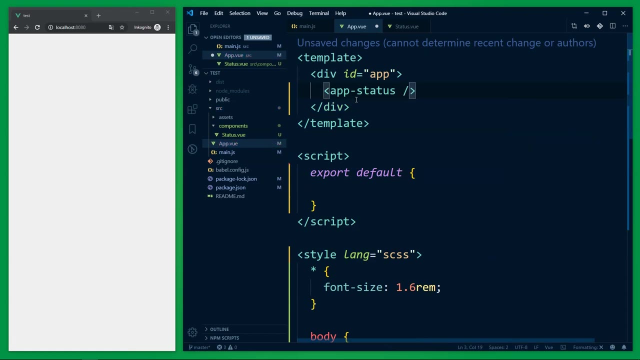 Now with this setup you can use app status as a selector in the whole application, Also in the root component appview. So I set app status in the template section And if I save now you can see here the button and the output right next to it. 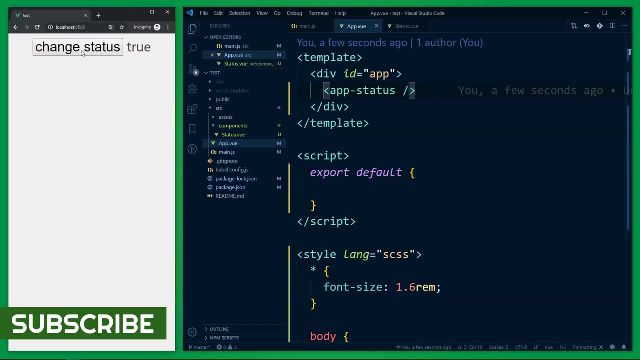 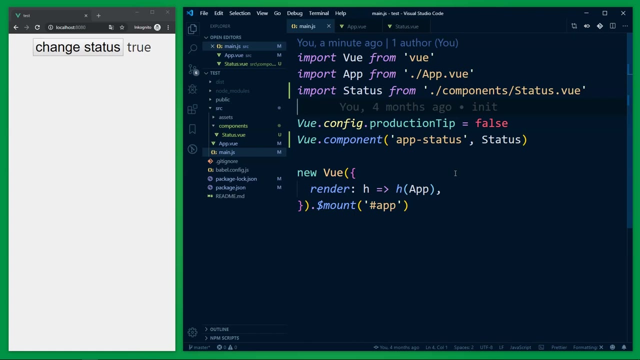 Now with this, if I hit the button, the status is changed. great Now, this is one way you can register a component Globally in the mainjs file. There is another way you can register a component. Imagine Your application is getting bigger and bigger with many components. 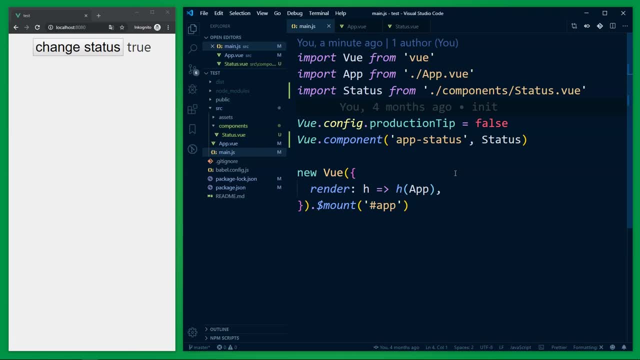 And every single component would have to be registered here. That can be a bit too much here. Additionally, you don't need every component everywhere, And if you need a component in one place only, you can register it in the root component or in another component you need. 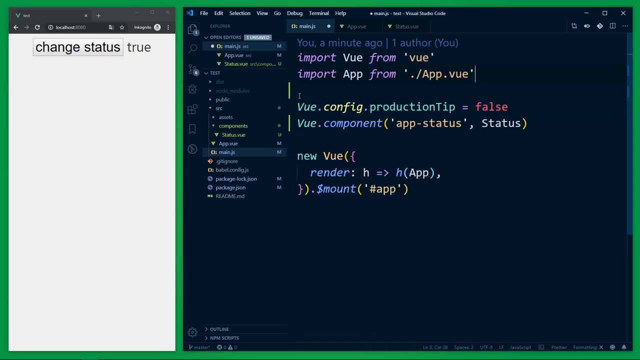 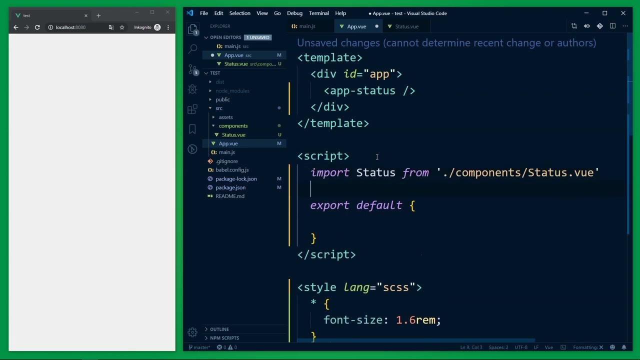 So You can cut out this import Here In the mainjs file, Remove this global registration here And put the import in your appview file Between the script tags here. But that alone will not work. View provides for this- a new property for us. 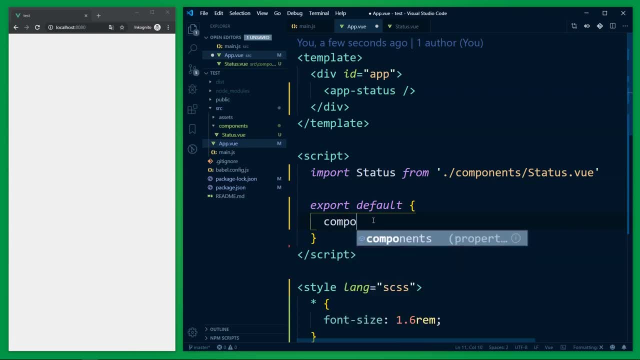 Simple named components Which holds an object, And here you can define your selector And, as a value, the name from the import. By the way, if you don't want to write a selector here, you can simply write here, in this case, 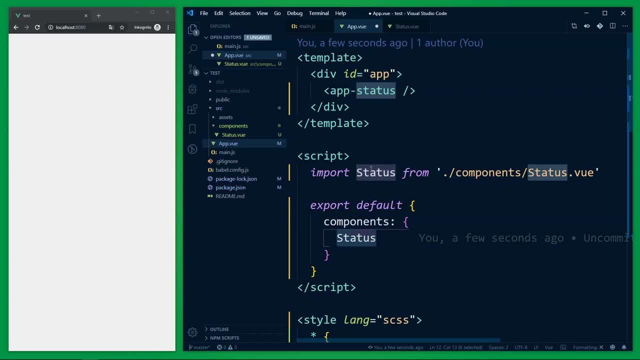 status And if you use in your template simply status as a selector view, match automatically this selector to your component which you are defined in the component object here. That's it. If I save, you see no difference. it still works the same as before. 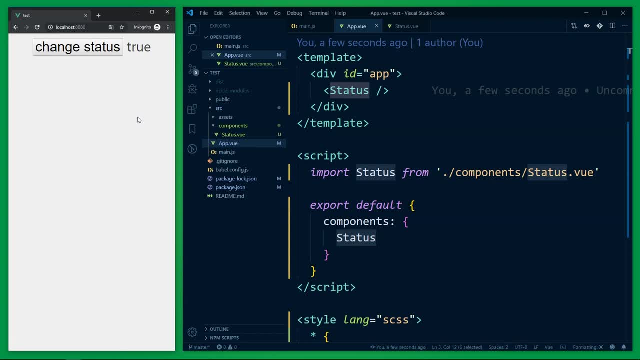 Ok, you remember a few minutes ago I talked about that you can re-render this same kind of code, in this case the component now in different places. So let's do this. You can use now this status selector here multiple times. 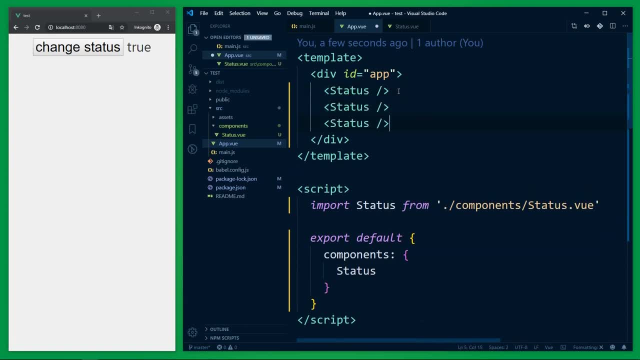 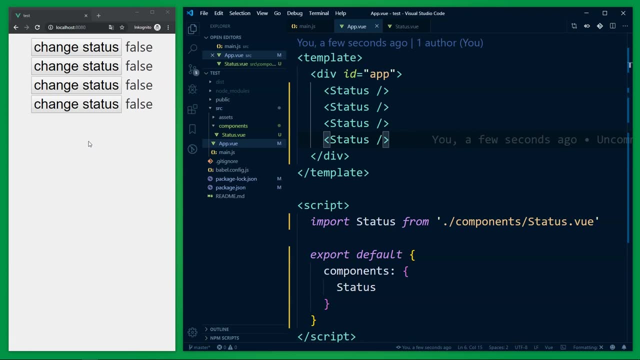 So I erase this a few times And if I save again, you see that the component is rendering multiple times And each component has its own status and functionality. This is how you can use components. Now let me show you a problem with the styling you can eventually have with components now. 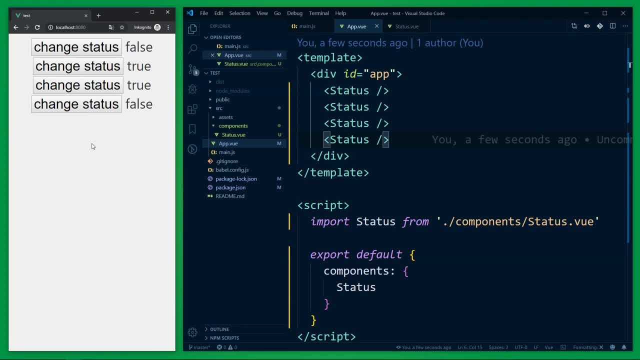 In this example, we have two components: The appvue file as root component and the status component, And each component has his own style. Now remember, in one of my last videos I say that the Vue CLI service is using Webpack under the hood. 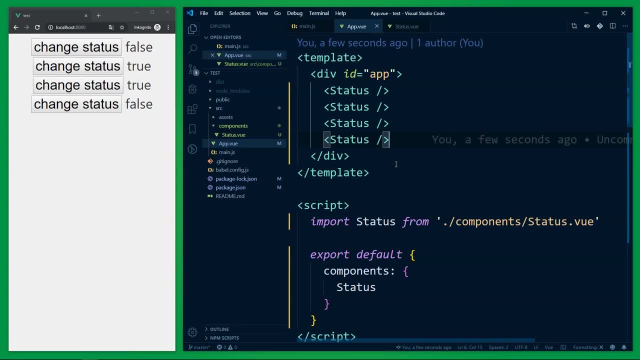 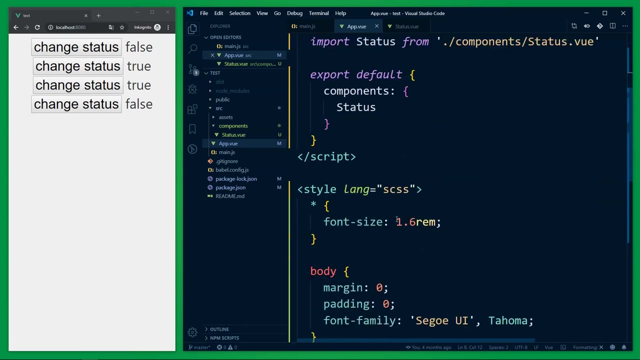 And Webpack merge all the code in one file, in the end also the CSS style, And if you use the same CSS elements in different components, Then the elements override each other. Let me show you this problem with a simple class styling. Named title.